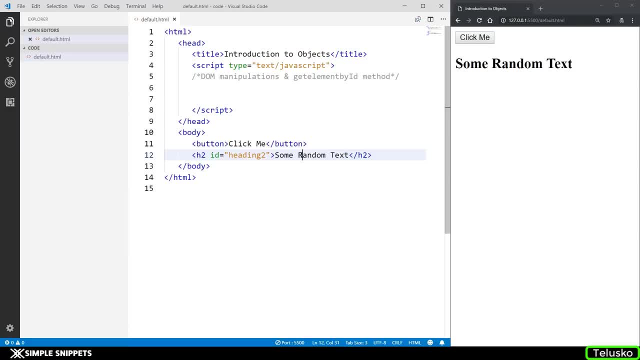 or you don't want them blank, or you want to perform some actions on some click events, then you can use JavaScript. So when you're talking about HTML document which is loaded onto the browser, there are a lot of events that are happening, So event is basically an activity. Let's say I am clicking this button, So this is an event. Okay, so you can have many standard events. So we have a lot of standard events in HTML, like click events, scrolling events. let's say you are changing focus from one text box to another text box, you're dragging some text, you're 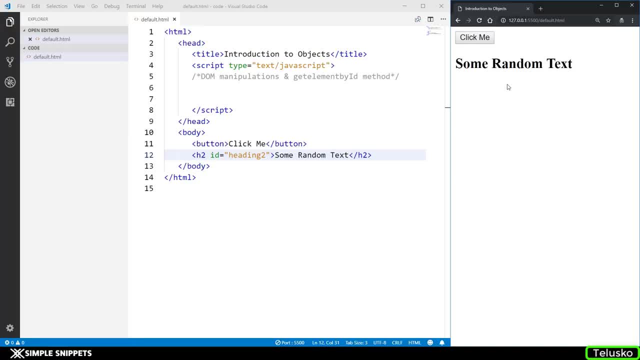 selecting something, you're double clicking on it, and so on and so forth. So there are a lot of standard events. I'll try to list some of them in the video description if you want. But then what happens is these events can be mapped into the JavaScript And we can target these particular events to perform certain actions. So in very basic, let's say you want to perform something when you click this button. So right now, if I'm trying to click it, nothing is happening. And also, by the way, I've zoomed in on the Chrome browser. the actual size is something like this, but then it will be very small in the 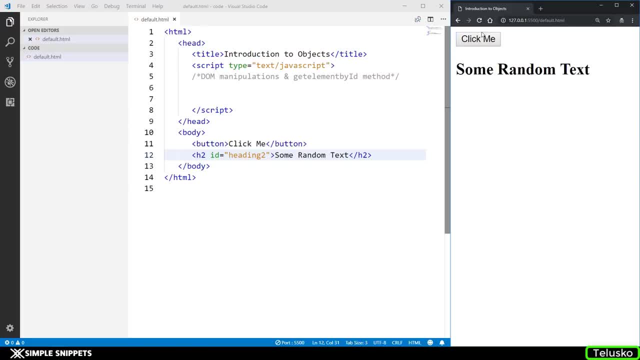 video right. So that's why I've just zoomed in a little bit. But yeah, what we want to do is, when we click on this, we want to show an alert message. So we need to actually map this event right. So, whenever we are clicking on this, something in the code, that is, something in the JavaScript, has to register this and we have to perform some action onto it, right? So this is where the DOM manipulations come into picture. So let's go ahead and add some functionality on this button. So in the HTML tag we have this button And, as I mentioned, we have some standard events which are related. 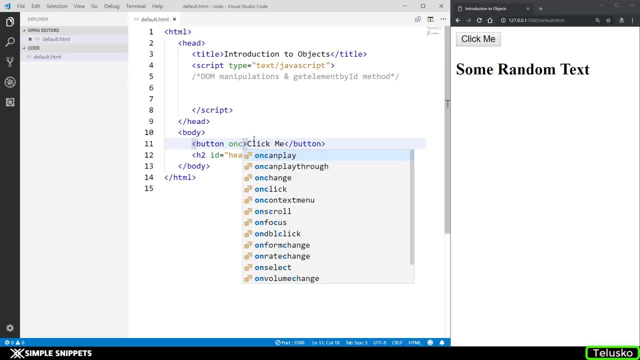 to HTML tags. So one of them is on click. So if I just type on and you can see that there are n number of events, actually these are all events that are showing up And we want the on click one. So I'm just going to click on it And there you go, the code is already generated for us. So the way we map these events to JavaScript is by using functions. Now we've already seen what are functions, right? Functions are a set of statements that perform a particular task And you can call them right. So you define a function and then you call it. So let's first actually 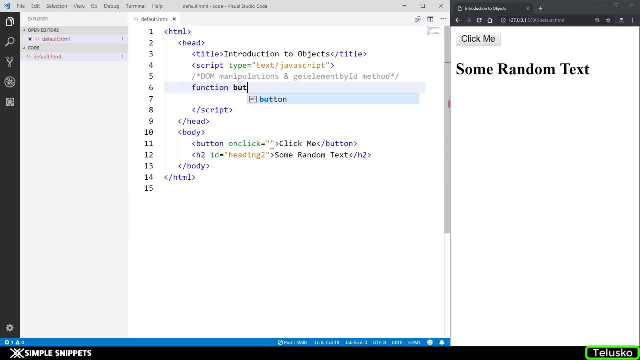 define a function. So I'm going to say function: button click. Okay. so this is the name of the function: opening and closing round brackets and the body. So this is something that I'm doing in the script tag. Okay. So I'm just defining a function And I'm going to say alert, which shows a pop up message. you'll see that in a minute. we've actually used it in the previous videos also. So this alert is a predefined method or function, And in the double quotes I'm just going to say button clicked. 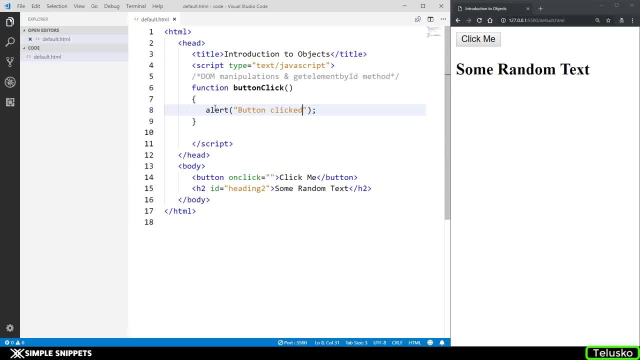 Okay, I'm just going to save this And you can see that I'm not really calling this anywhere as of now. So if I just call this over here, you can see immediately in the output we're getting button click. but we don't want this right. We are not wanting to call it immediately, We want to call this method when the button is actually clicked. So again coming back to this event of the button tag, So what we do is we just write the function name over here, So you say button click and opening and closing round. 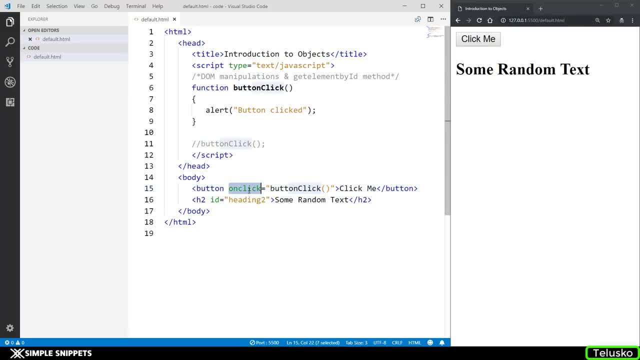 brackets of the function. So now what we just did is we registered this on click event to call this JavaScript function, And we've defined our function over here. So whenever I try to click on this, so if I click now, you can see button clicked, So we're getting that message. So what we just did in a very simple way, is we added functionality to this button. right, We made it do something when we wanted it to do it. So, essentially, this is something that we are going to be doing a lot in the further videos wherein we are going to be mapping certain events to certain functions. 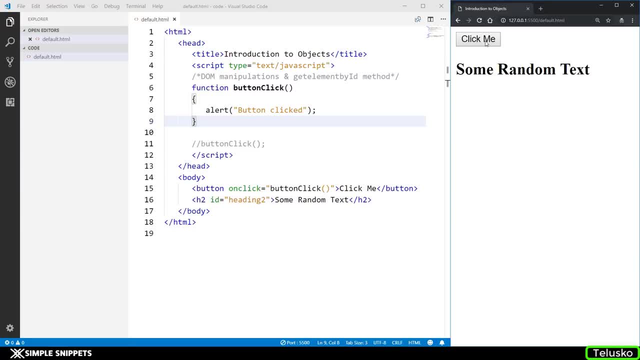 And we're going to be performing certain activities, what we want. Let's say you want to perform validations. let's say you want to perform animations. you want to perform, or you want to change the CSS styling of some text, you want to change the text, and so on and so forth. So this was just the mapping of events. Now, just let's talk about the get element by ID method. Now let's say you want to perform something else on this button click. you don't want to show this alert, But what you want to do is you want to change this text and type in something else, right? Let's say you want to type in telescope learnings, But 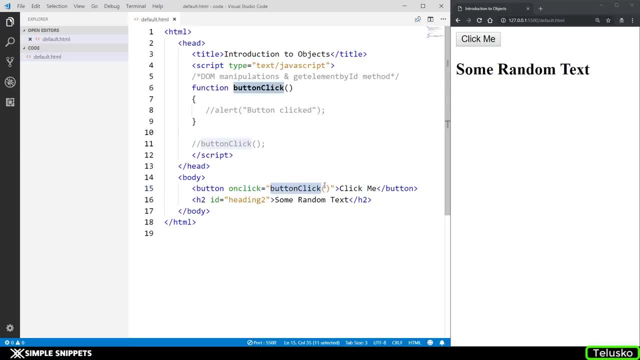 this should happen only on this click. So the button click event is going to be the same. However, the function code, that is, the statements inside the function, has to be different, right? So what I'm going to do over here is I'm going to say document. Now, document is a predefined object. If you've seen the document object model, you know that the document object represents the entire document that is loaded into the browser. That is the HTML document. And using this document object we can access certain predefined methods and functions. So here what I'm going to do is I'm going to say document dot. I'm going to say get element. 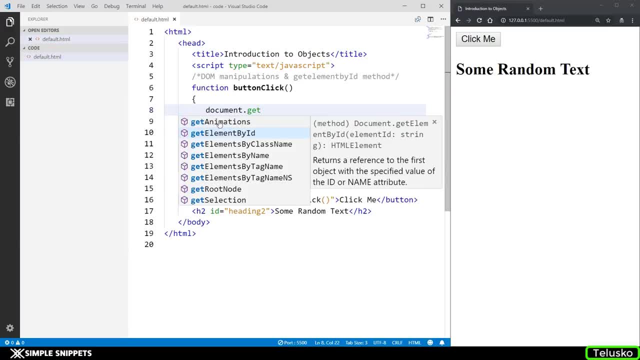 by ID. So what this method does is you can actually read: the definition also returns a reference to the first object with the specified value of the ID or the name attribute. So I'm just going to hit enter and opening and closing around brackets. and inside this, around brackets, what I'm going to pass is: I'm going to pass the ID of this h2 tag. So this h2 tag has this unique ID, heading two. Okay, so I'm just going to copy this, I'm going to paste it over here. So, essentially, what we're doing is: 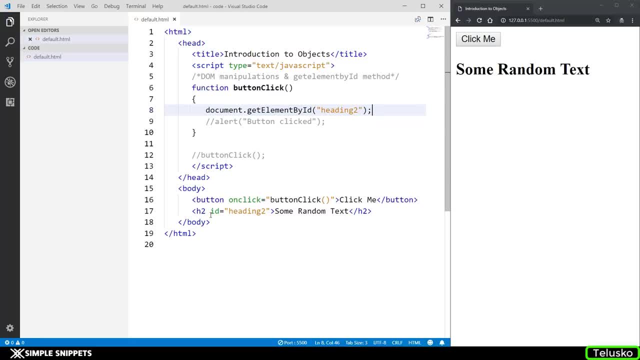 we are trying to fetch that element on the web page whose ID is heading two. So, using the document object, we are trying to identify which tag or which element has this heading to ID. So we know that h2 tag has this right now when I access this. so basically we are getting a reference right. so you can see why the definition also returns the reference of the element which has this particular ID or name. right now it is ID. Now, once I get the reference of this h2 tag, because h2 tag is represented as a 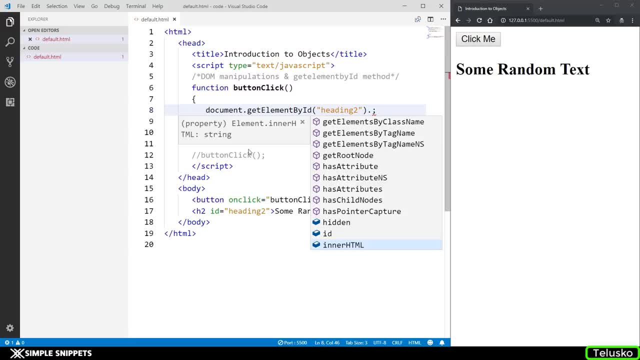 object in the document object model, I can say dot and then I can say inner HTML. So inner HTML is a property of the h2 DOM object, because this h2 tag is represented as an object, right? so JavaScript sees it as an object. So objects has properties. That's what we saw in the objects video. So inner HTML is a predefined property of this h2 tag, of this basically element that we just found out, And this inner HTML property is actually the text which the tag holds. Okay, so if I say equal to,